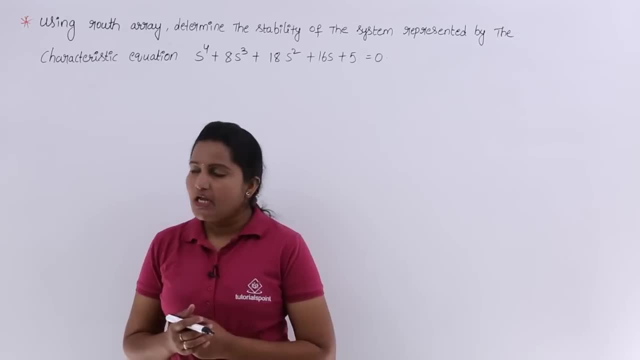 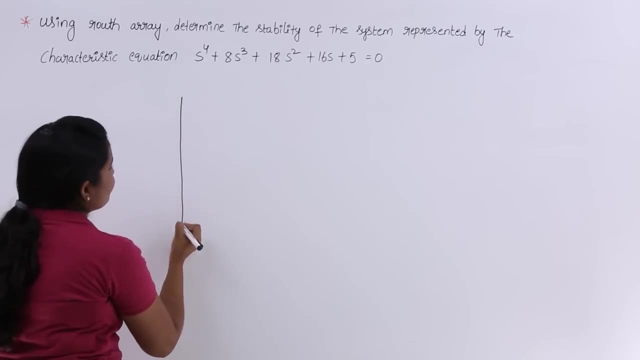 we need to justify the condition of stability. So to frame route array, we need to consider a line like this, and after that we need to consider: from maximum power of s to minimum power s power of s. that means up to s power 0, s power 4, s cube s square s power 1 and s power 0 up to s. 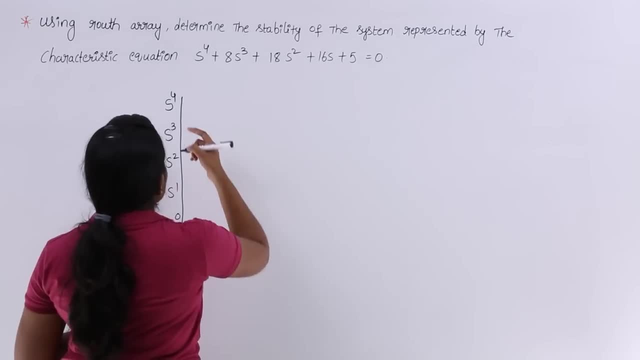 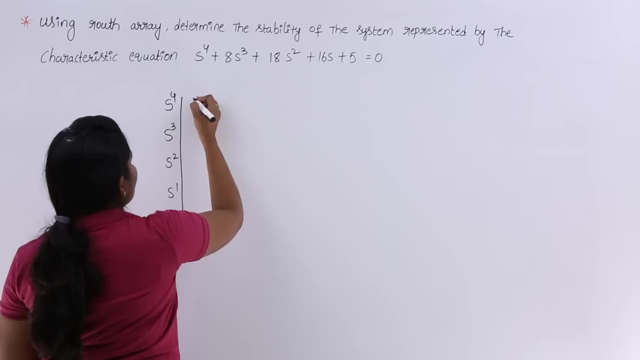 power 0 we need to consider. And here s power 4 means here you need to consider. so here the coefficient is 1. we need to consider like this: So if this is a 1, a 2, a 3, a 4, and this is a, 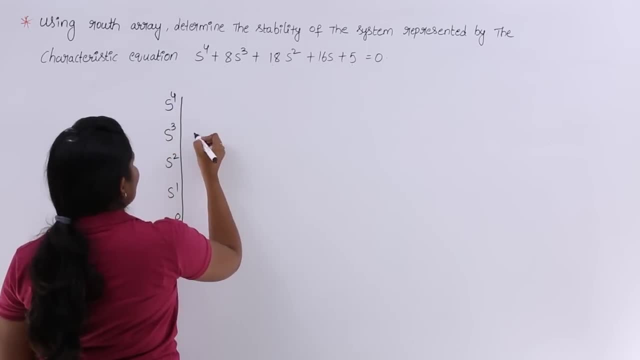 naught. So you need to consider like this: a 1, a 2, a 3, a 4, a 5, a 6. like that we need to consider in first two rows. So that means 1, 8.. So 1, 8,, 18,, 16 and 5.. So over up to here. 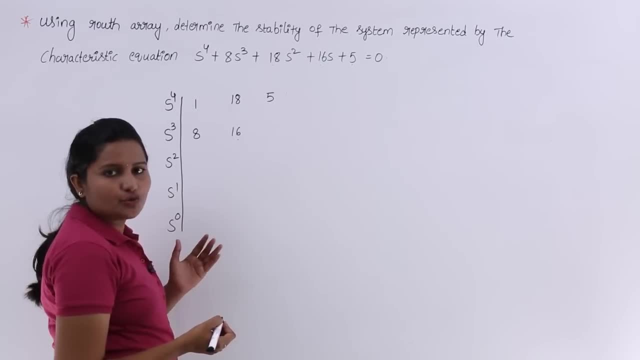 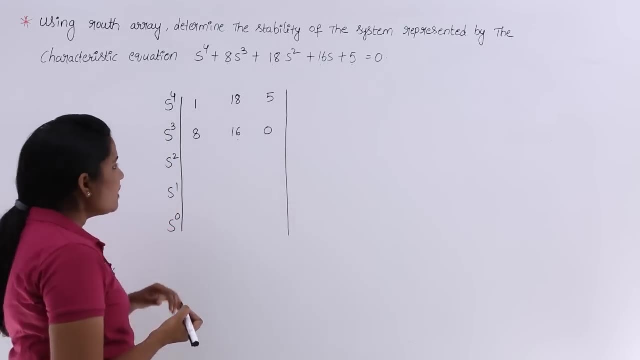 the values are over. So what we need to do here means so we need to put 0 and we need to close this Routh array. Remaining values we need to find out from the previous values came from this characteristic equation. For example, if you want to get this value, then you need to do like this: So 8 into 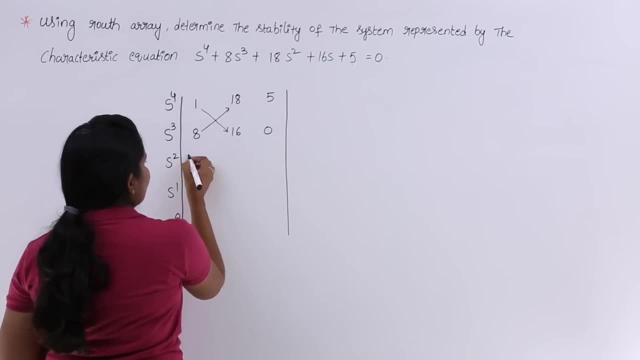 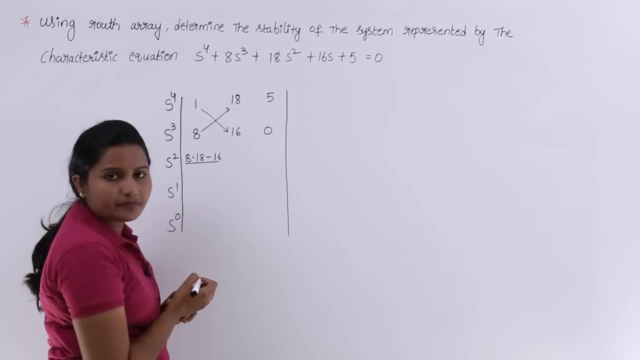 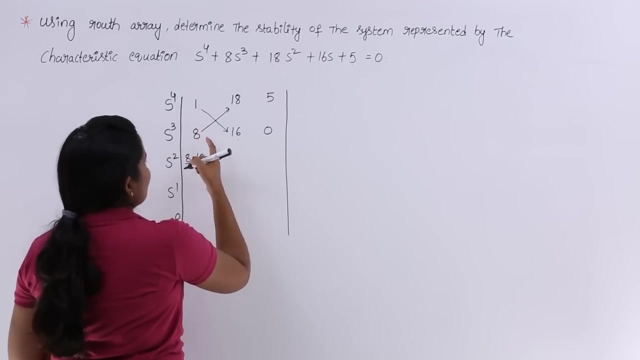 18 minus 1 into 16 divided by 8. that means 8 into 18 minus 1 into 16 means 16 divided by So 8. we need to consider like this And after that. So here you can see. So if you want to get this value, So you need to consider this set and this. 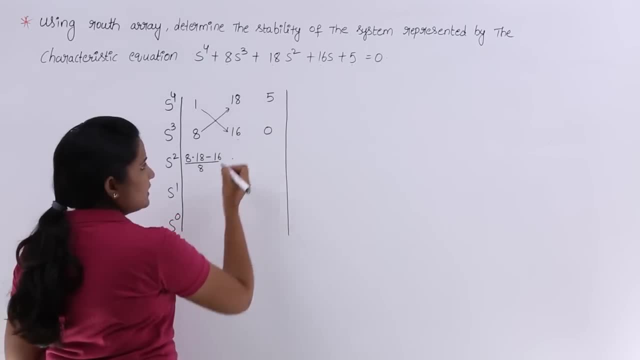 set. whatever the cross set to this point is there that you need to consider. So you need to do the same procedure which we done here for these two sets to get this value. So that means so here. So 8 into 5, 8 into 5 minus 1 into 0.. 1 into 0 means 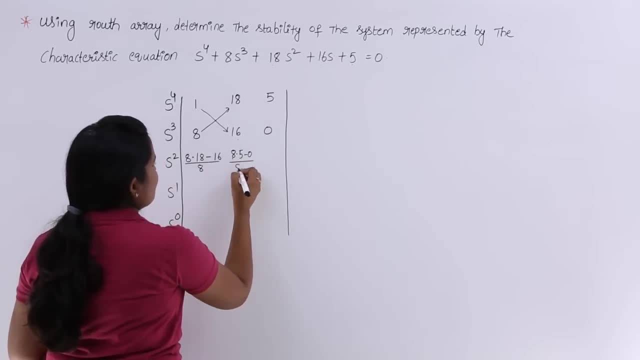 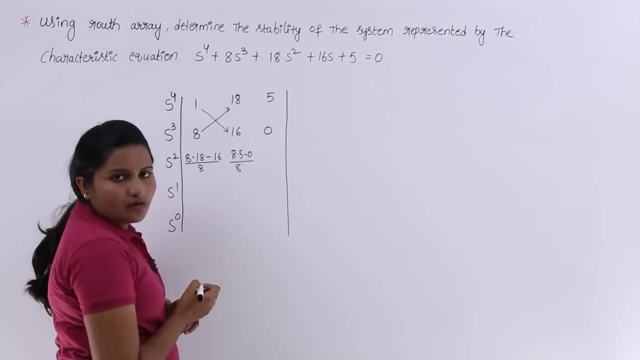 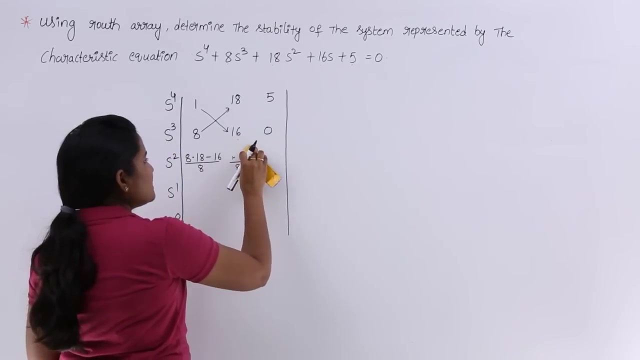 So you are going to get 0 divided by 8.. 8 into 5, 1 into 0 divided by 8, 8 into 5, minus zero divided by 5.. So here, so, so 8 into 5 means we can consider this as 40. so 8 into 5, 8 into 5, you are writing. minus 0 means. 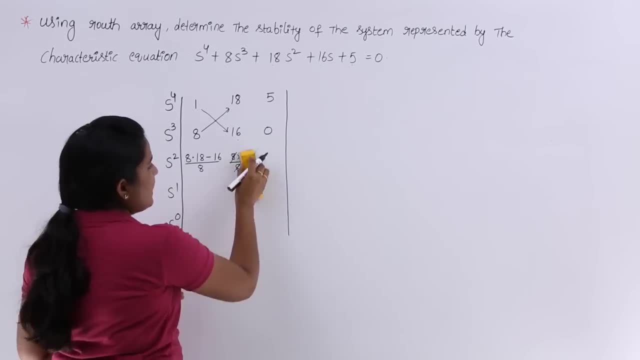 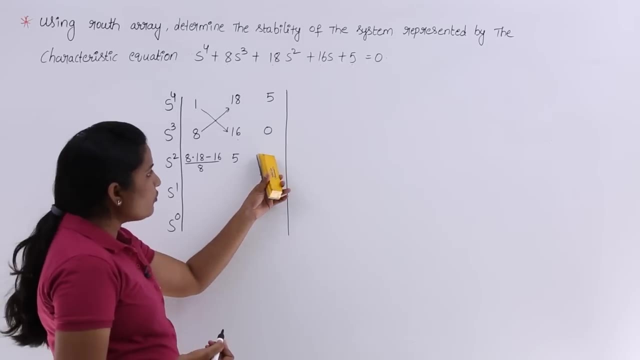 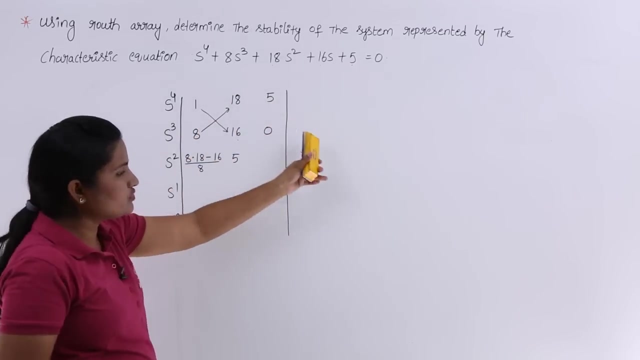 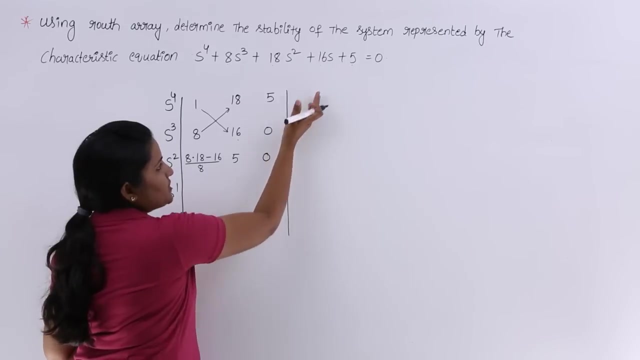 no need to consider 8. 8 will be cancelled and you are going to get 5 here. the value here is equivalent to 5 and if you want this value, as you are not having this set, if you consider 8 into 0, 1 into 0 divided by 8, you are going to get 0 only, as you are not having a crash set to this point. 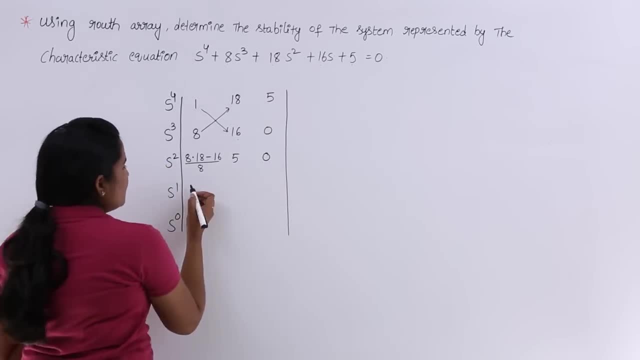 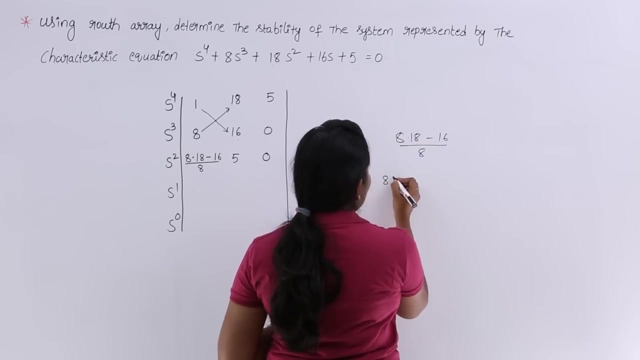 you are going to get 0 here and now. this is the time to evaluate this point. so now for this point, you need to consider this value. so here you can see this is a positive value or negative value. so i am taking common of 8 here. so here, if you want to evaluate 8 into 18 minus 16 by 8, if you want to take 8 out, 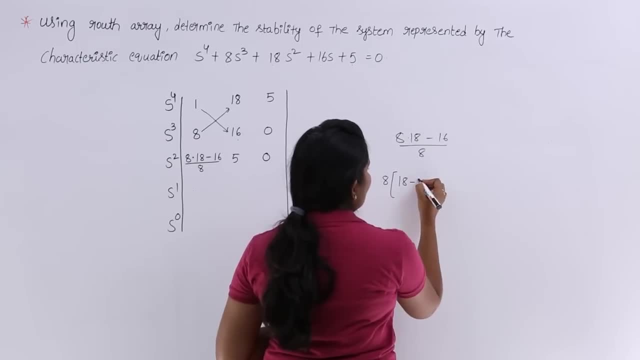 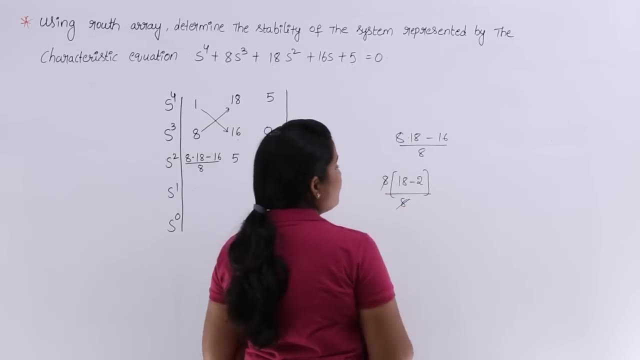 so 18 minus so 2, 18 minus 2 divided by 8, so 8. 8 will be cancelled and the remaining may be 16, right, so here 8 to 16. so i am taking common of 8 and cancelling with denominator 8. 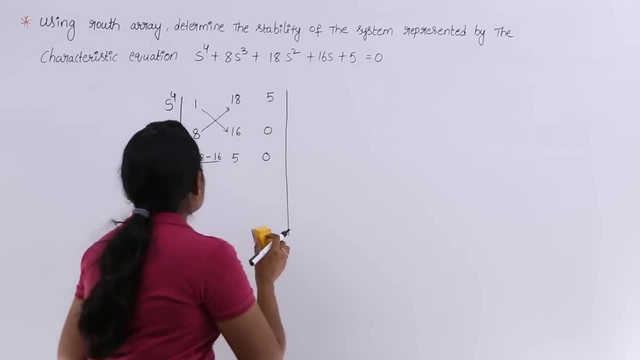 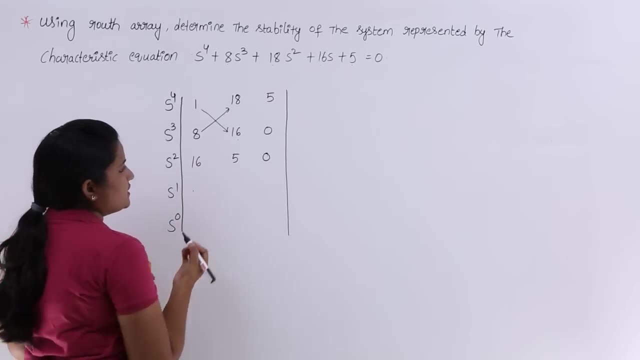 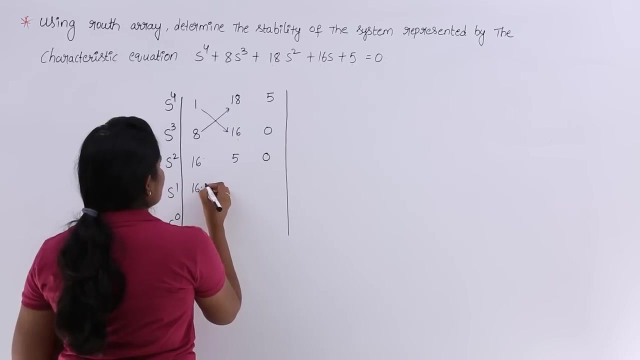 18 minus 2, you are going to get 16 here. So here I am going to consider 16. and now, if you want this point, 16 into 16, 16 into 16 minus, so 8 into 5 divided by 16.. So here, 16. 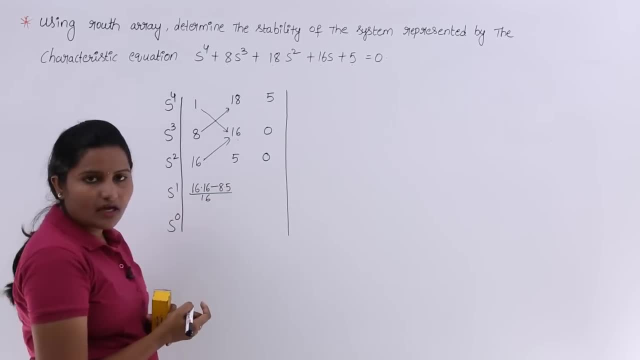 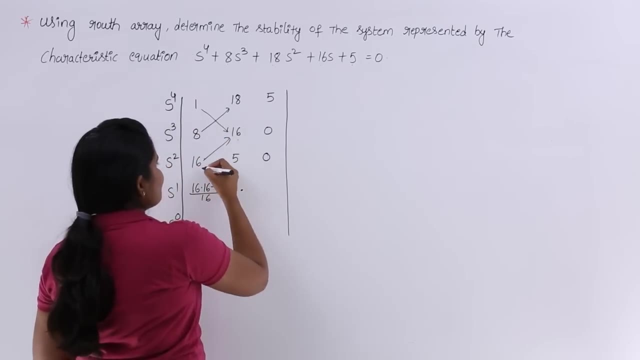 into 16 minus 8 into 5 divided by 16. I am considering like this and coming to this position: so how we will get 16.. We will get this position, this set, with this set, If you consider 18 into 0,, 16 into 0. 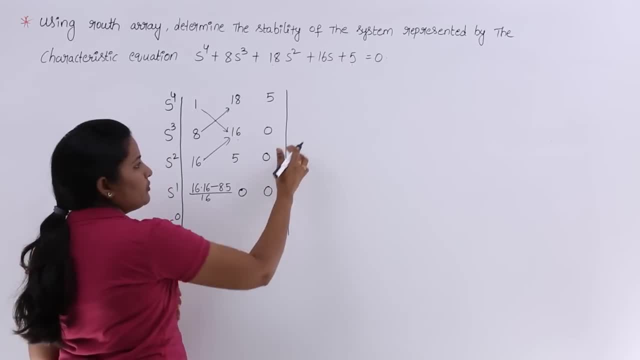 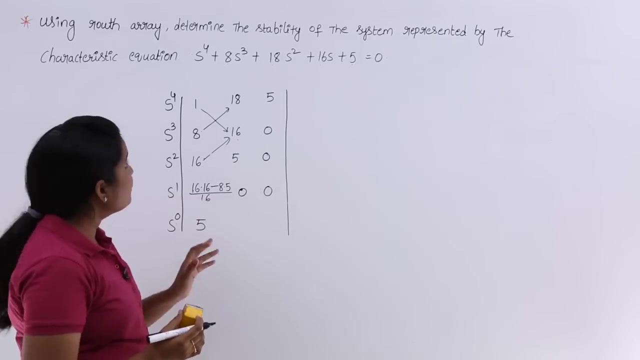 you are going to get 0. This position also. you are going to get 0 because you are not having cross set to multiply with this set. So now here S naught is always you need to consider the final value 5.. So here you need to consider EAL. If you observe the fundamental, 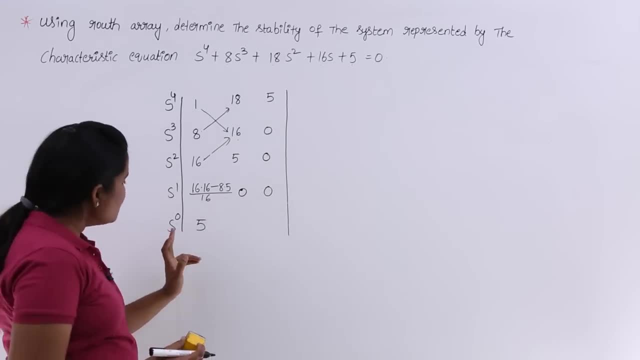 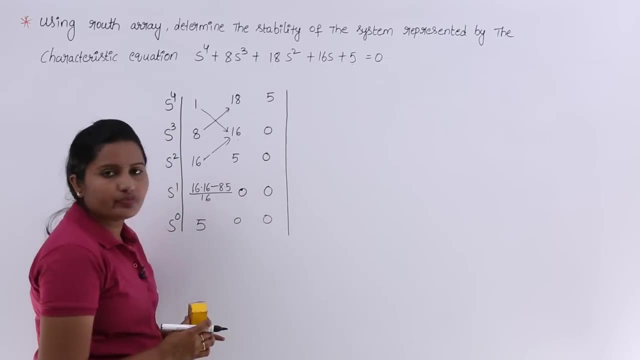 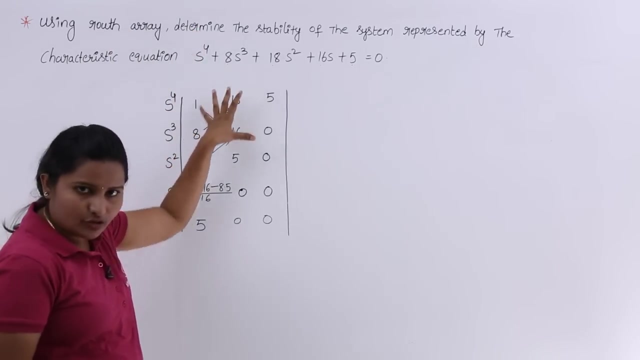 Routh array which I described. I discussed in the last class. So at S naught you need to consider AN. So remaining places, you need to put 0.. Now what we need to calculate what they are asking using Routh array. that means you need to form Routh array. After forming Routh array, determine the stability. 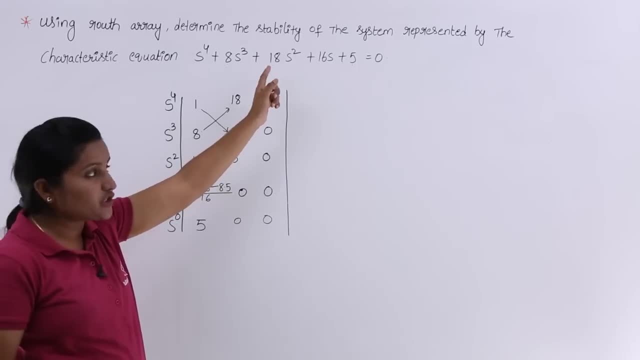 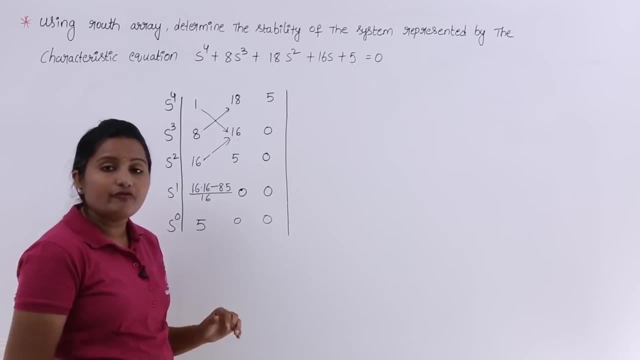 of the system represented by this characteristic equation. By this characteristic equation we formed the Routh array. From this Routh array we need to justify: the system is stable or not. we need to justify the stability of the system. whether that is stable or not, we need to justify here. So 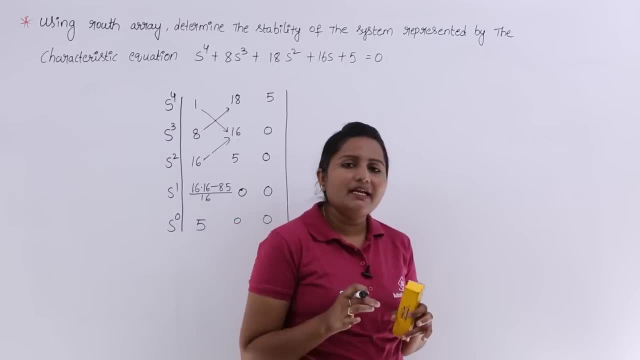 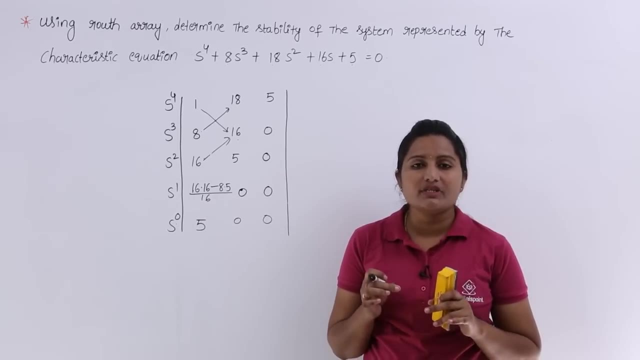 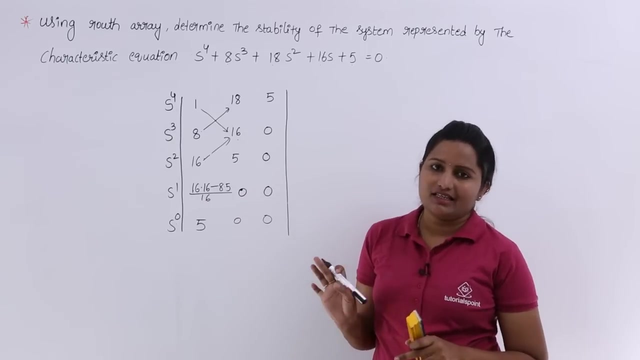 that means, if you see, what is this stability condition, what is the statement of Routh array means- this is very important condition- that a system to be stable, the first column of Routh array must be positive when A naught greater than 1.. Now, depression is a condition which is usually referred as an expression or phenomenon, or 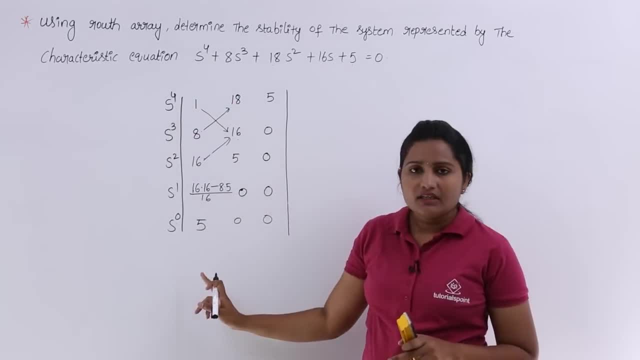 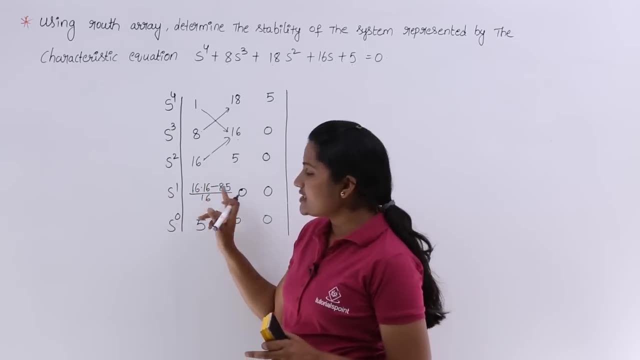 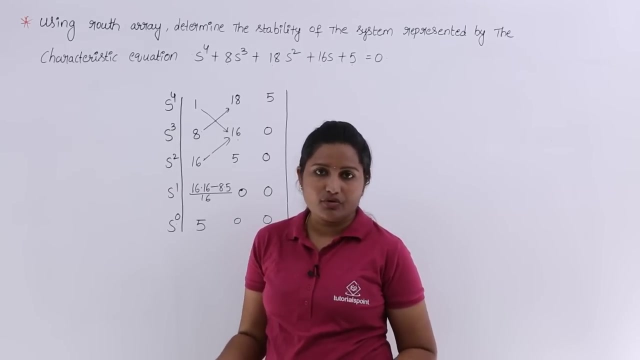 1, definitely a, not greater than 1. the first column must be positive to say the system is stable. you, if you see, 16 into 16 is very much greater than 8 into 5. so divided by 16 also you are going to get greater than 0, not less than 0. so definitely this is a positive. 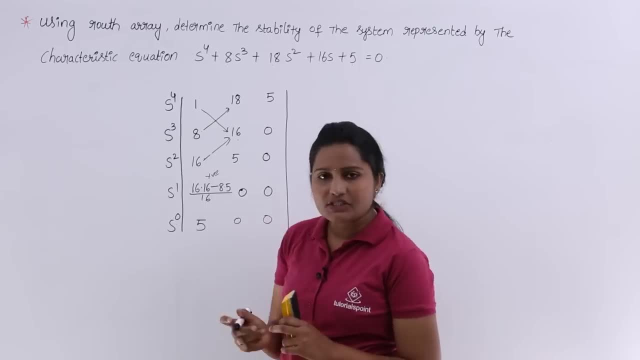 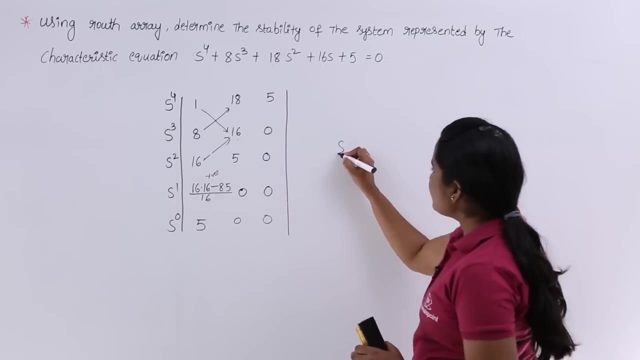 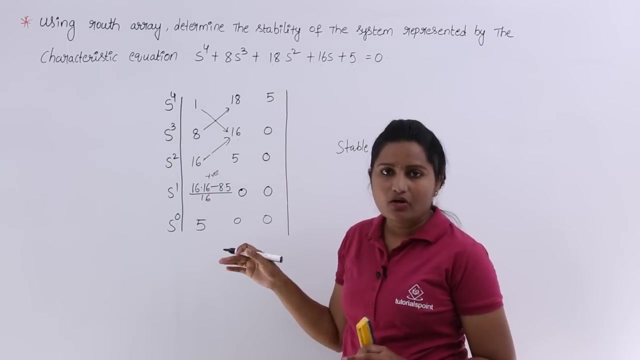 value and coming to all the elements in first column, all the elements are positive, then definitely we can say this system is a stable system. according to the routh array formed by the characteristic equation of a system, this system is said to be a stable system. why? because